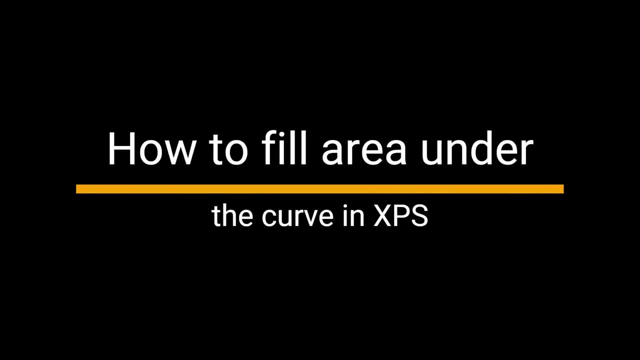 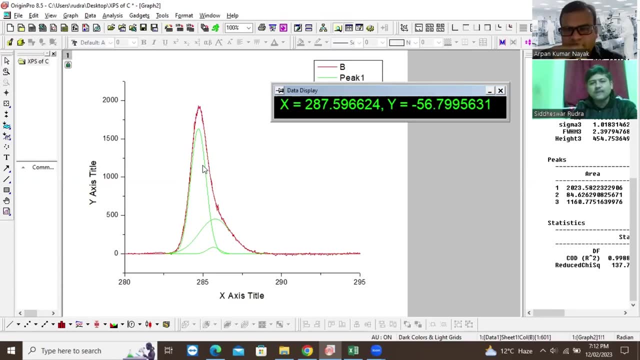 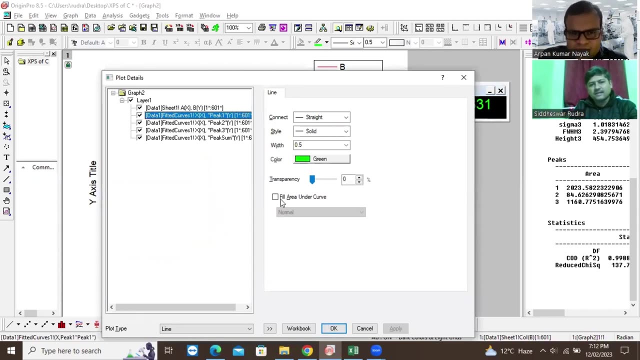 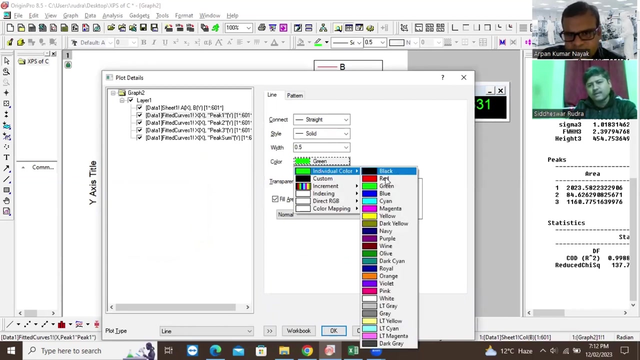 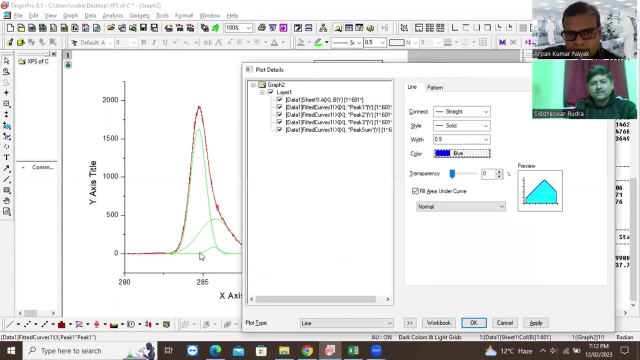 So you have to give the three different segments. Now you click it here, Okay, And there is the option lines and everything. You can change the color also. In the color we can put black, green, everything else, Whatever you require, And to fill this portion, we select the fill area. 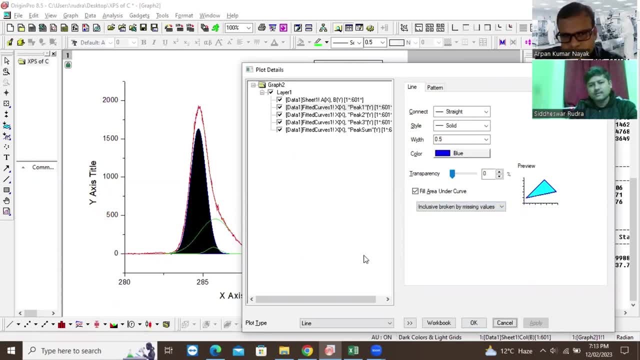 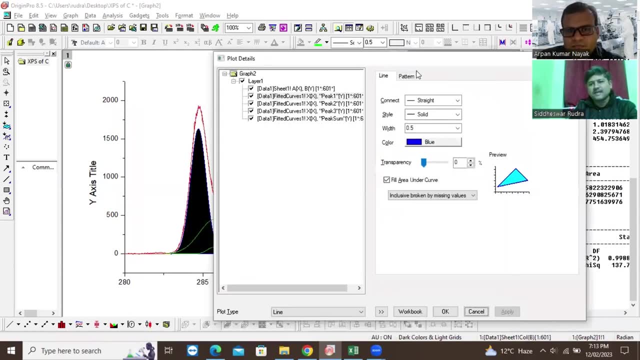 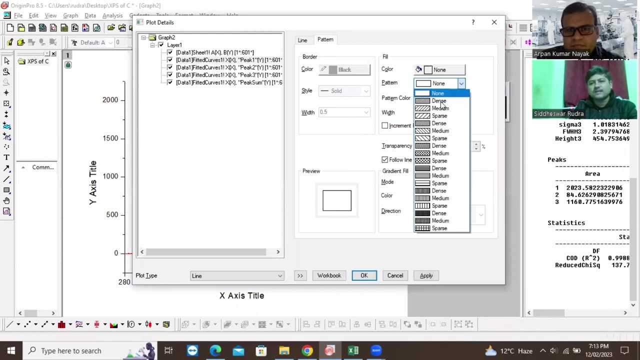 under the curve. Okay, Yes, And then we can change also this fitting color, also This pattern. you can give, suppose, black. if you give none, there is no color. If you give the dense and if you put the blue and if you change this thickness, width, actually to 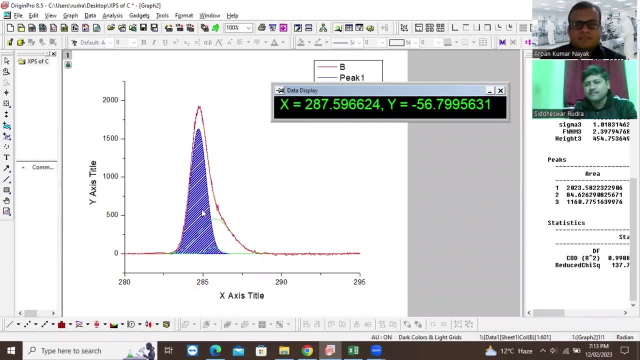 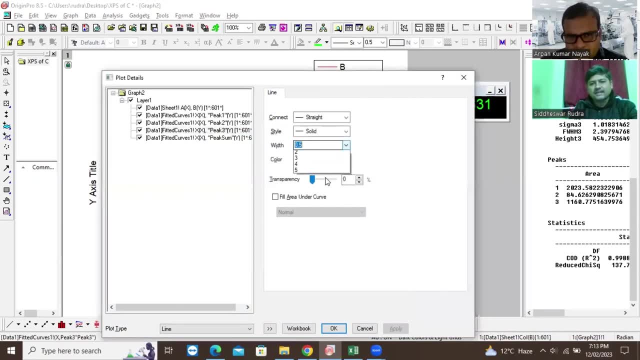 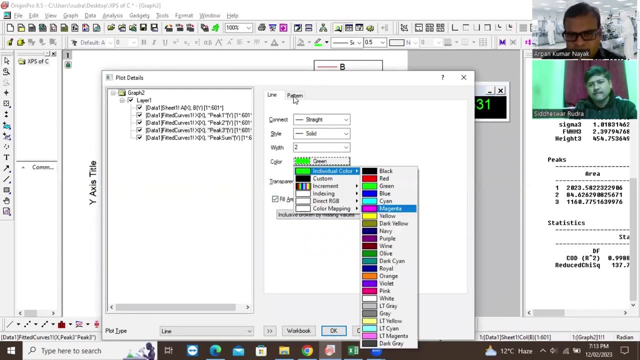 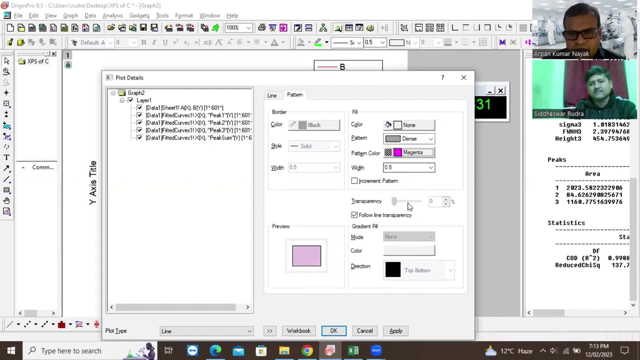 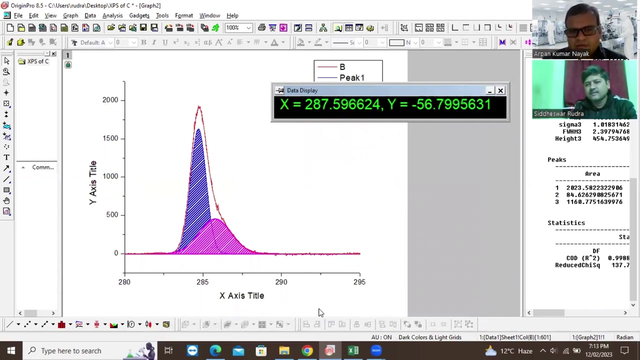 that will get the good looking curve, Yes, Okay, Yes, And again this curve also. if you put the another, another segments, another color, magenta- you can put the magenta and every dense and color also. If you put the magenta color, then we will see like that only Yes, Yes. And if we 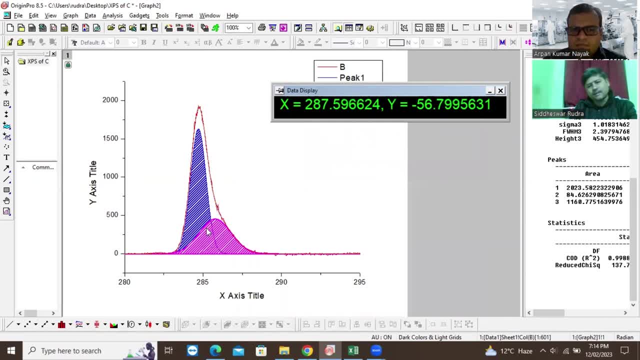 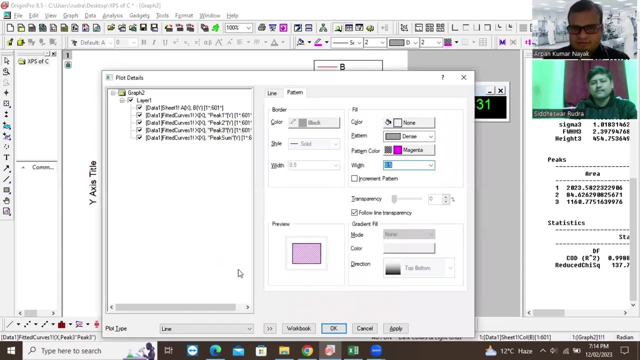 we can, we can, we can do anything from the color changing. We can do any color, We can put any color, No problem, And the light color also is given. If you change the thickness, we drop the color. If you change it to see this point, 0.5.. Yes, Then see this one. 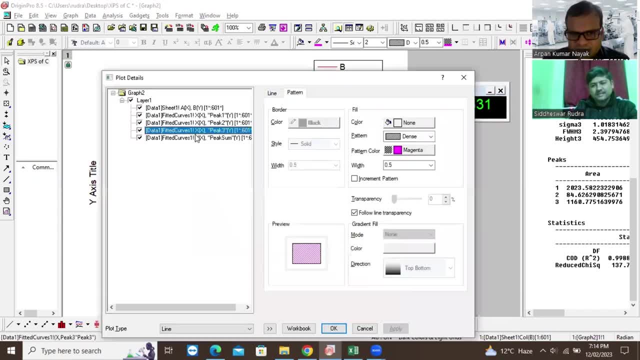 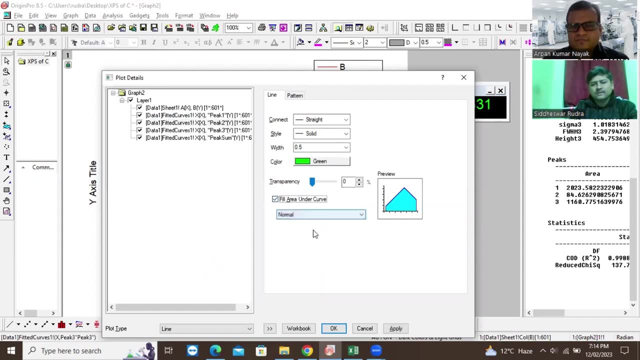 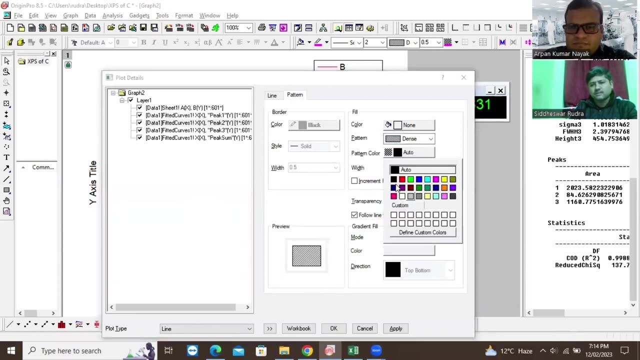 Right, And now the p. third peak is there. Actually, third peak, is there? This one? This one fit in the curve If you give the another color. so now see what will be the black color. we choose the black color, the more prominent. this magenta, I think.